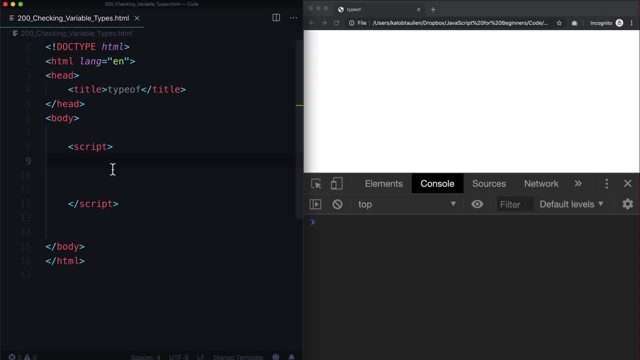 a string, or an array or a number. Now, behind all of these different types of variables is a thing called a data type or, in some languages, a data structure. So let's go ahead and look at a few of these. So let's create var. age is equal to 30.. Okay, we know. 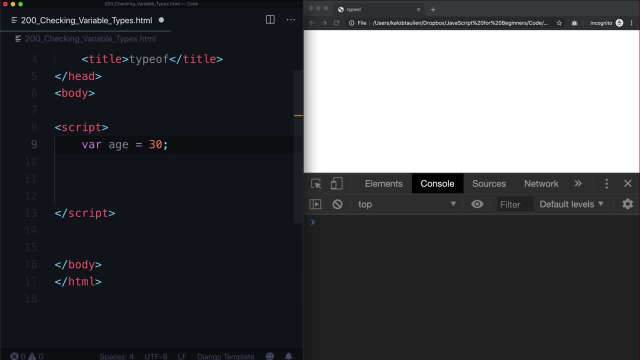 that this is a number, but what does JavaScript think it is? Does it think it's a string, a number, anything like that? Let's create another one in here. var name is equal to JavaScript. for beginners, What does JavaScript think? this variable is Var. you know, we. 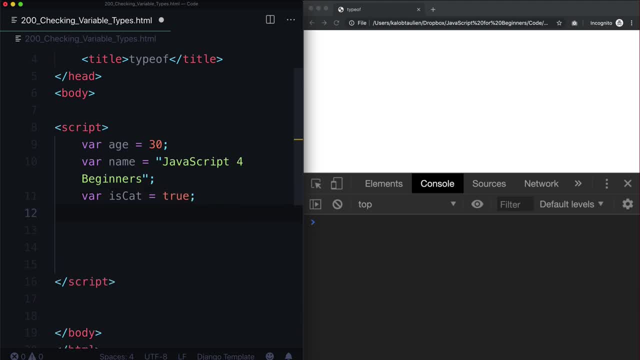 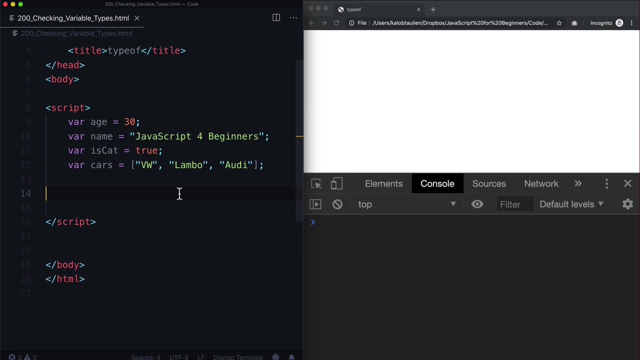 did this one already. Is cat true or false? And let's create one more. Var cars is equal to Volkswagen Lambo and Audi Audio Audi, Something like that. Let's, yeah, let's put that all in one line again, And so when we refresh our page, we're not going to see anything. 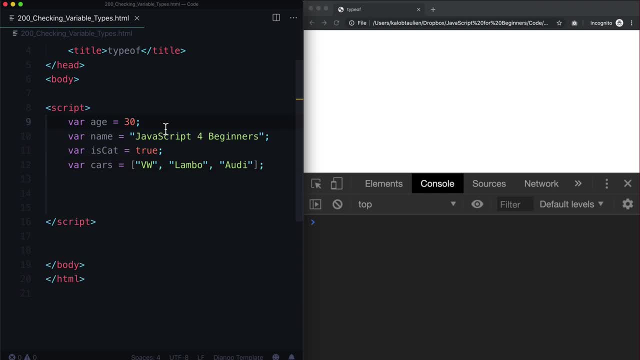 happen. We've declared a bunch of variables, but we're not doing anything with them. Let's go ahead and consolelog each one. So consolelog age is, and in here we're going to use a function called type of, And it's just simply going to say age is, and then we're going. 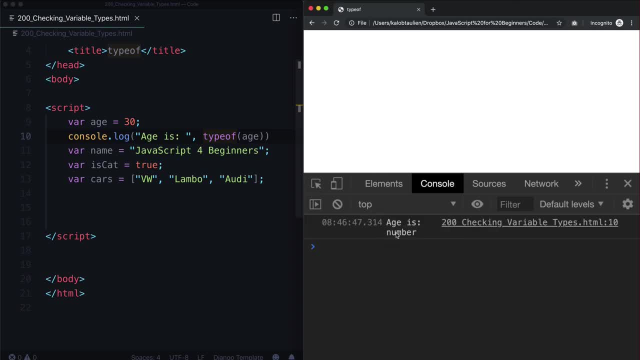 to see what it actually is. So let's go ahead and save this and we're going to see: age is a number, That's the variable type Or the data type. Let's go ahead and create another one in here. Say the name is the name of this course, is whatever that's going to be. 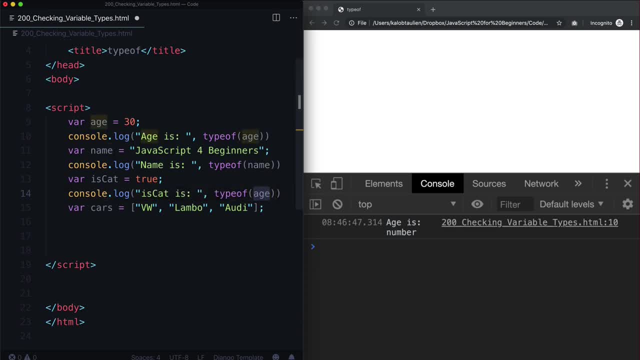 Is cat is going to be, Is cat. And lastly, we have cars is Cars. Okay, so, before I Refresh my page- Actually I'm going to make some space here so that this actually looks somewhat legible- We know that age is a number. JavaScript told us it's a number. What do? 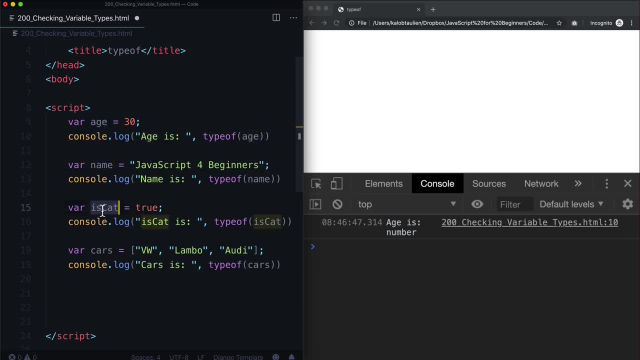 you think name is, And what do you think cat is, And what do you think cars is? We have at some point gone through all of these, but we haven't actually fully explored their data types. I mean, we sort of have in a sense, but not completely. So if I hit refresh, 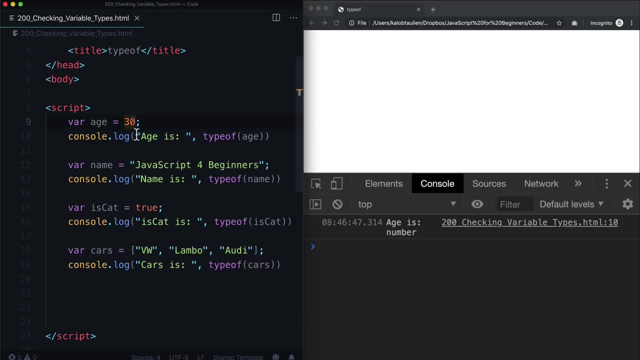 on this page. I'll save this and hit refresh. We're going to see that age is a number, name is a string, is cat is a boolean and cars is an array. So age is a number, name is a string is cat is a boolean, cars is. 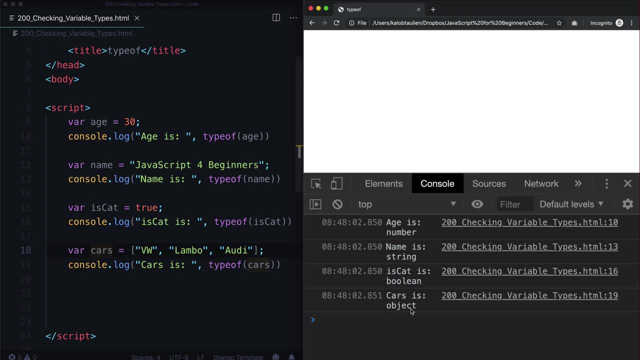 Oh, what's this? It's not an array. Hmm, Well, that's interesting. Even though we told it to be an array, it's actually this thing called an object And, interestingly enough, even if we do this Do-do-do-do-do-do-do, Let's go ahead and change this to the word array. 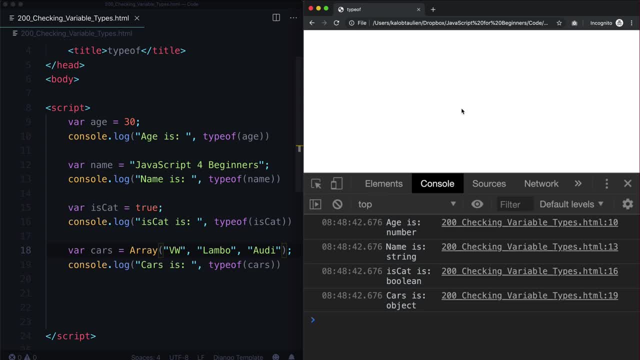 We're going to see that this does not change. I hit refresh and it still says cars is an object. What is with that? Well, in JavaScript and in many other languages- object-orientated programming languages- we have this idea of an object, And an object really is just a. 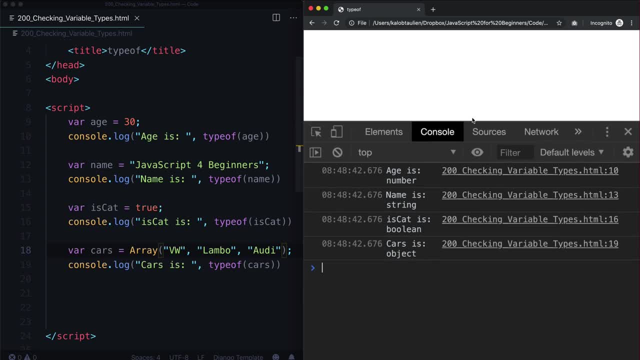 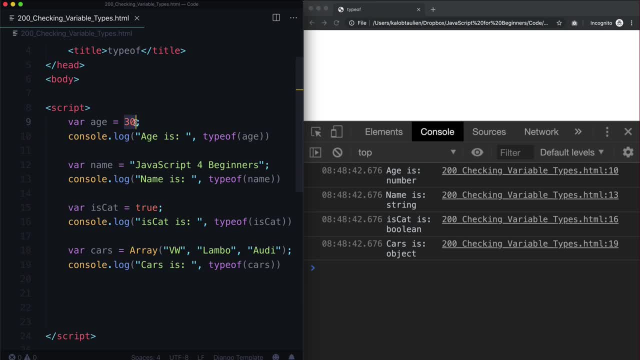 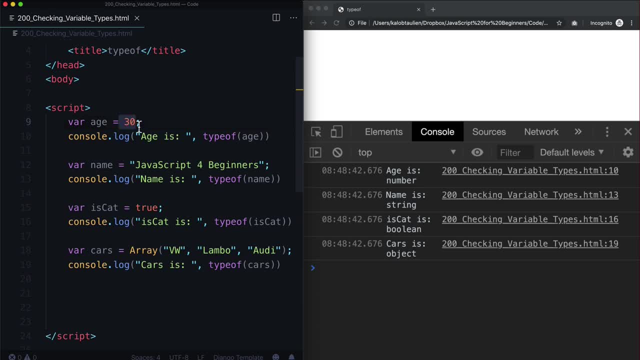 the last item, Because there's only one item in here. It's not even a list or an array. We can't really do anything with that. We can't add too many custom functions to it, It's just a number, Whereas with the variable called cars it's an object And we can actually 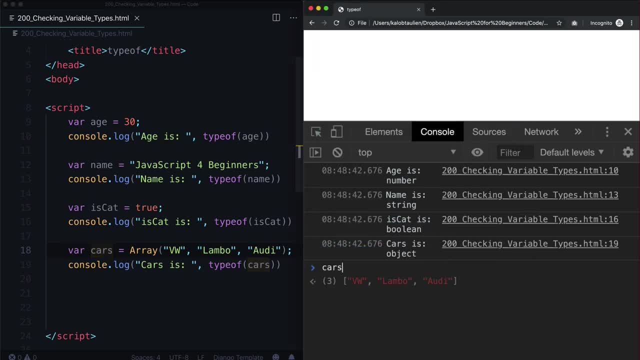 do a lot more with objects, So let's go ahead and take a look at this real quick Cars dot and all I have to do. you can see that it says concat array. here is hit dot, and, and just scroll down and you can see all these different things that I can perform. 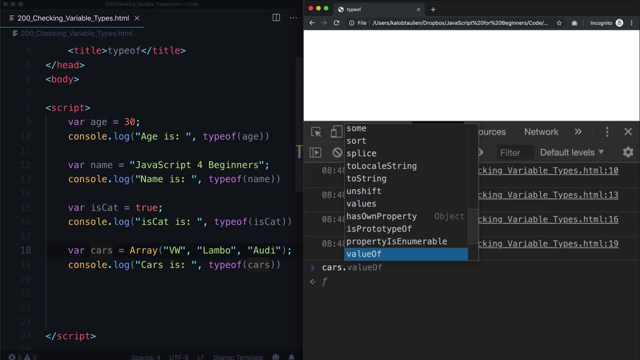 on this particular type of object Now. we're going to get into objects much more in depth down the road, So you don't have to worry about knowing the difference between an array and an object right now, Because, yeah, we'll totally cover that in this course. But the thing that 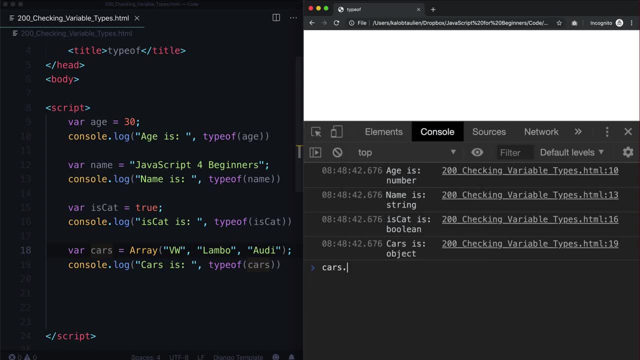 I did want to make you aware of is different data types. using the function type of, we could type cars and it gives us an object. Now, why is this important? Well, let's take a look at the difference between one particular property. So if we did agelength, well, we don't have agelength. 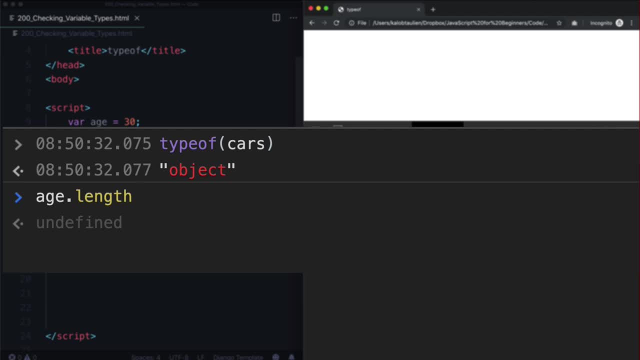 That's because it's a number. There is no length to a number. Well, I mean, in human terms there is, but to a computer there is not. It just says: oh, it's a number. I mean, what do you want from? 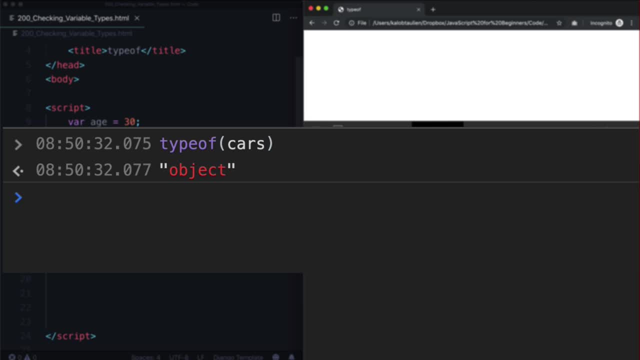 me, The number is the number, And so numbers are pretty basic. If we said namelength, we know that this is a string. If we did namelength, we know that this one is, in particular, a string, So it's going to count. 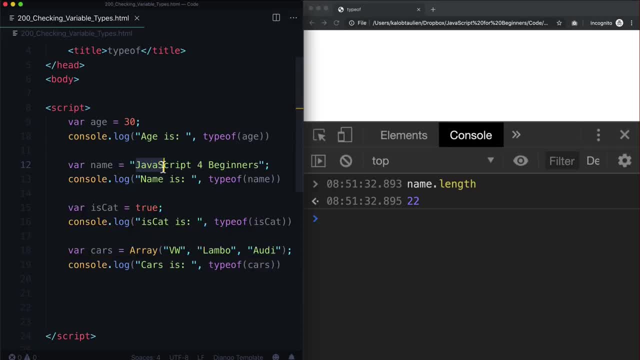 the number of characters in it. So J-A-V-A-S-C-R-I-P-T, space four, space B-E-G-I-N-N-E-R-S: 22 characters. Now, what if we did? is catlength Undefined? It doesn't even have a property called. 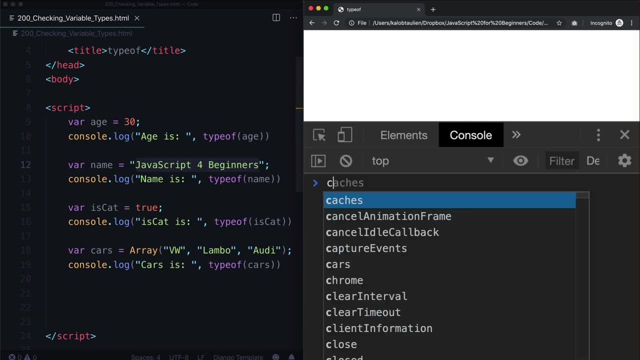 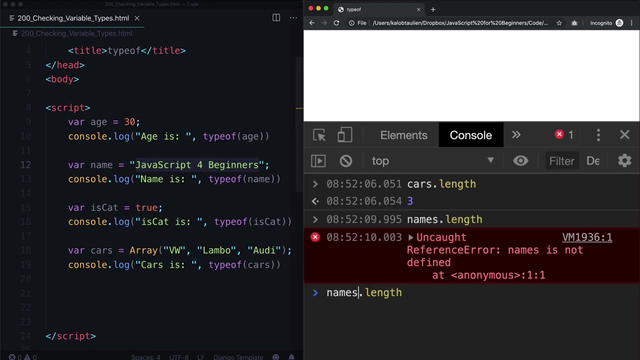 length, We can't use that, But with cars, because it's an object or, as we currently know it, as an array, we can do length and this will return three. Where this gets important to know is if I did that wrong, if we did, if we did carslength, we're going to get three as the total number of cars. 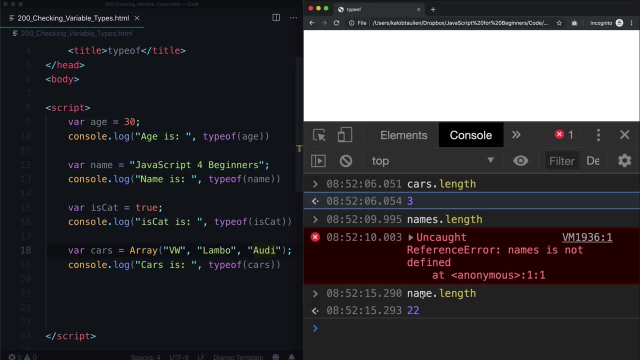 We've got Volkswagen, Lambo and Audi. But if we did namelength- ignore the one that I messed up there with the typo- If we did namelength, we're going to get three as the total number of cars. If we did namelength, we're going to get the total number of characters, And so that's very. 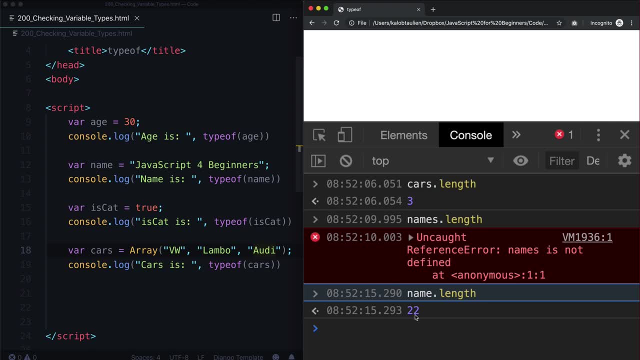 different. And so if you try to do length on a string versus length on an array, you're going to get different answers And that might change your logic down the road. You might say: if the array has five names in it, do something, But if your logic says if variable length is equal to, 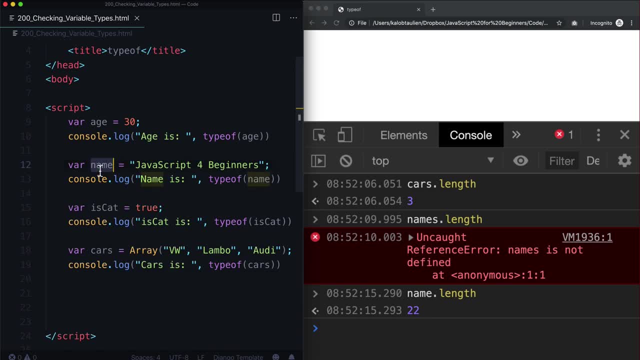 five and someone just types in a word with five letters in it, that's also going to trigger, And so that's sort of the difference between data types is, you know, some of them have certain functions or properties on them that we can use and some of them don't.